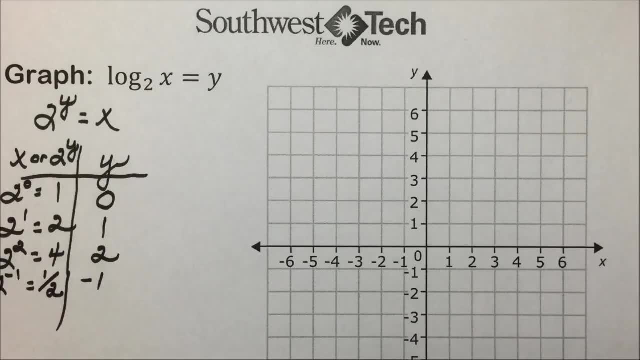 1 would put that exponent in the denominator to make it positive. So it would be 1 over 2 to the first power or 1 half. If we let y equal negative 2, we would have 2 to the negative 2 power, which is 1 over 2 squared or 1 half. 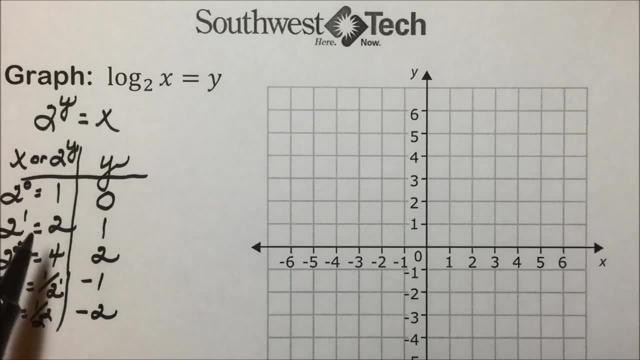 So we have 2 to the fourth. We have enough points. Let's plot those points. And even though we started with y, our ordered pairs are always x, y. So we'll plot the point 1, 0,, 1, 0.. We'll plot the point 2, 1.. We'll plot the point 4, 2, so over 4 and up, 2.. We're 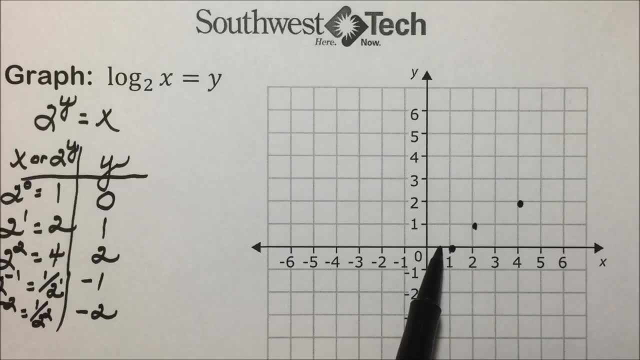 going to plot the point 1, half negative 1,, so halfway and negative 1.. We had 1, 4, and 1, 4 when we simplified here is negative 2, so 1, 4 is negative 2.. And if we connect, 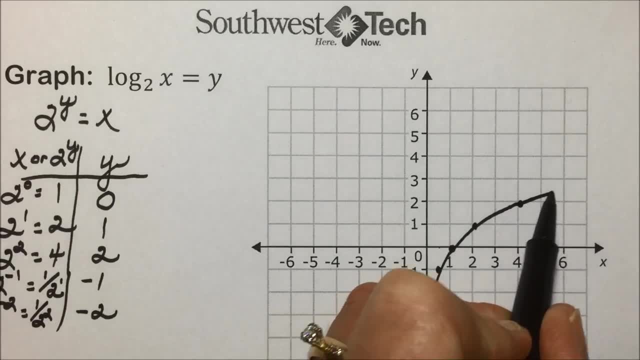 those points with a smooth curve. we've seen something very similar to this earlier. This is the function that we're asked to graph, but using the definition of a logarithm or a logarithmic function. they are the inverse of the exponential function. 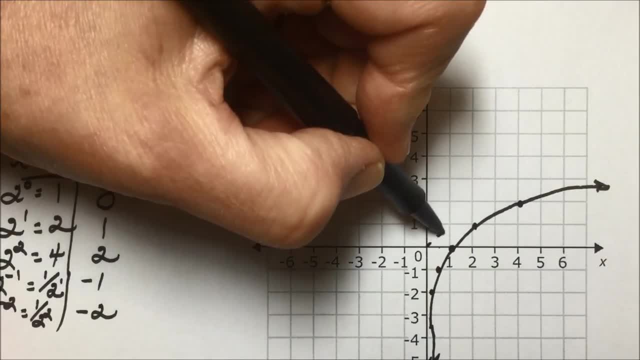 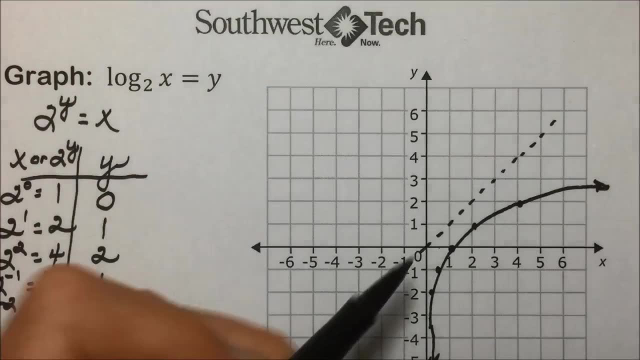 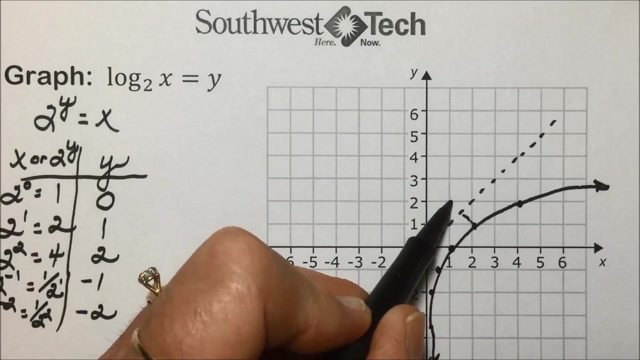 So, just for reference sake, if I graph the y equals x line and I reflect these points about that line, this point 2, 1 becomes 1, 2. when we reflect it through there, The point 4, 2 becomes 2, 4.. This point here, which is 1, 0, becomes 0, 1.. Our half is negative. 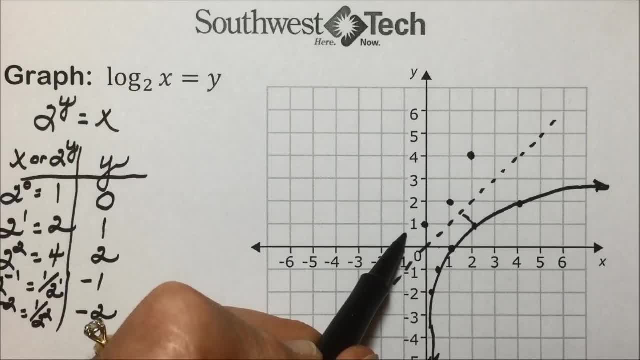 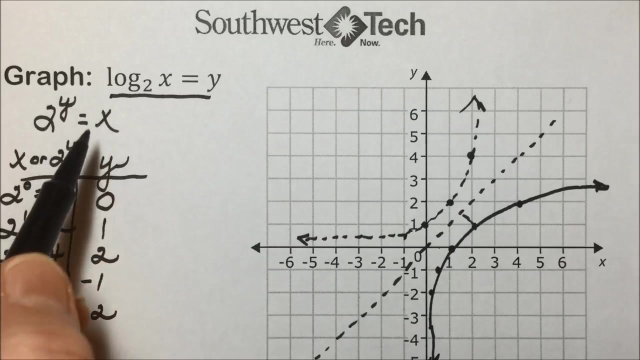 1, 1 half and so on. And if we do a smooth curve here, we end up with the reflection or the inverse of this logarithmic function. And if we investigated this further, we would end up finding that the inverse of this logarithmic function is actually 2, 2, 0, 0, 0, 0, 0, 0,.